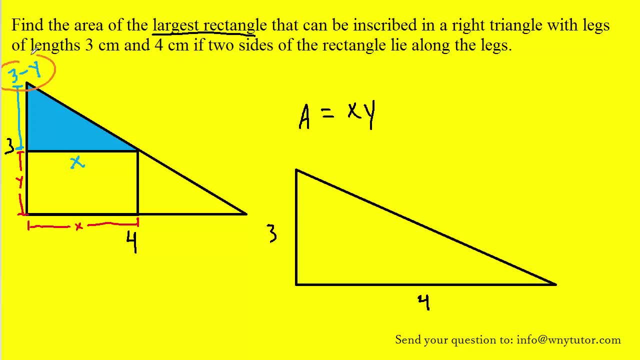 triangle here, and thus, because they're similar, we can write a proportion. We can say that this side, this 3 minus y, is to x, As this side- 3, is to 4.. So let's write that proportion right over here. What we'll do next is solve this. 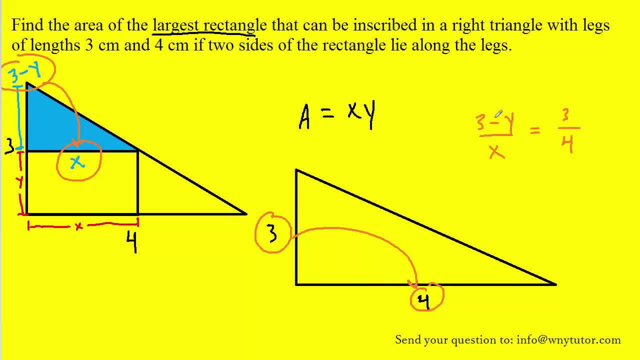 equation for y so that we can substitute into our original equation. So to solve this we'll have to first cross multiply, We'll then divide both sides by 4, subtract 3 next, and then divide both sides by negative 1.. So let's take this expression for y and plug it into our original equation, and that'll be nice. 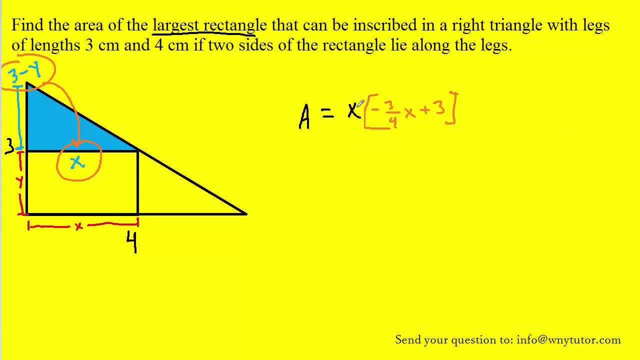 because then we'll have an equation with just a single variable in it. To simplify this equation, we can distribute the x into the brackets And then, since we're trying to find the largest rectangle, we're trying to optimize. in other words, we're going to have to take the derivative of both sides of this. 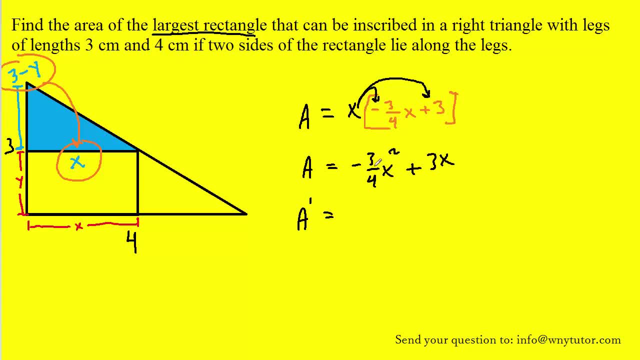 equation, The derivative of the area we can symbolize as just a prime. The derivative of the right side will incorporate just a few basic rules. We'll use the power rule to drag this exponent down and multiply by the coefficient, so that'll give us negative 6 fourths. 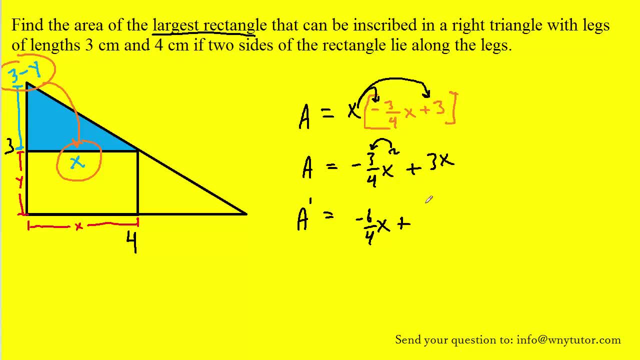 x, we'll subtract 1 from the exponent to just give us x to the first, And then the derivative of 3x, of course, is just 3.. Next, we're going to have to set this equation equal to 0.. Maybe we could subtract 3 from both sides. 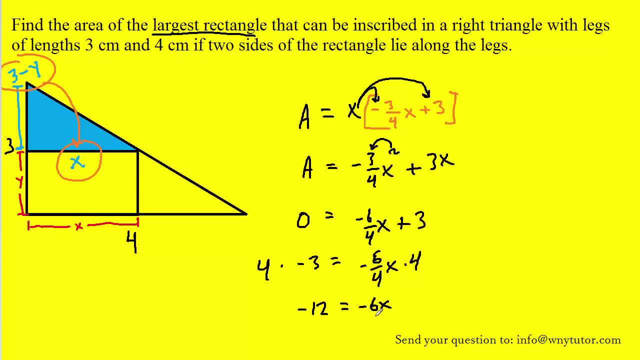 Let's multiply both sides by 4, and then divide by negative 6. And we get x equals 2.. Now, technically, in order to ensure that this is a largest rectangle, we'll have to do the first derivative test to make sure that this value of x is. 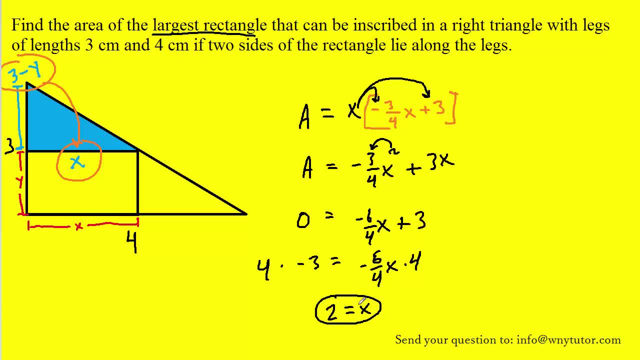 indeed producing a maximum value for the area. So let's do the first derivative test, And we can do that by plotting 2 on a number line. What we'll do is we'll choose a value less than 2, such as 1,. 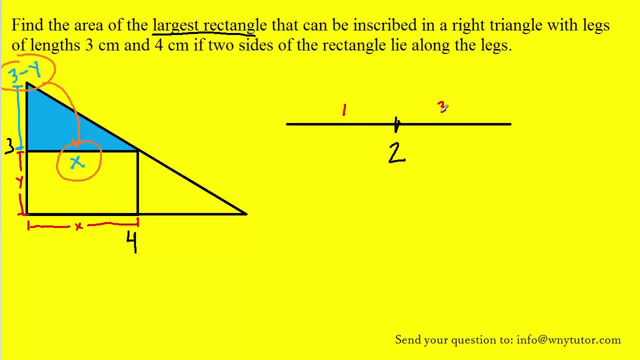 and a value greater than 2, such as 3, and we'll plug them into the first derivative. Let's bring the first derivative back into the picture here just as a reminder. Now, if we plug 1 into the first derivative, we get a positive result, So we can say that the derivative is positive.